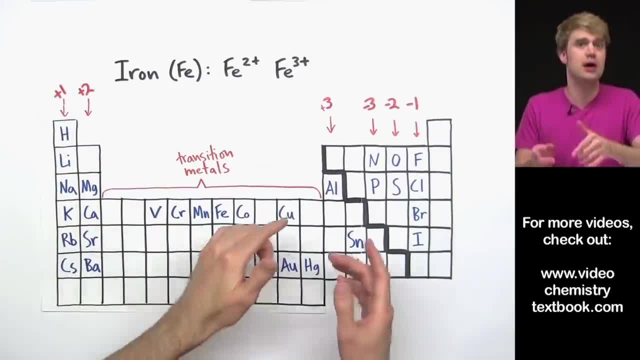 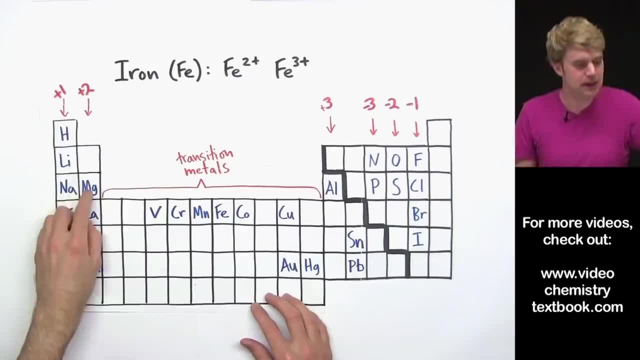 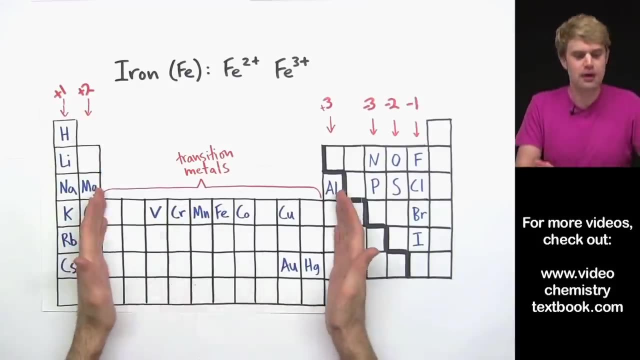 plus one column here, and so when sodium is in an ionic compound it always makes an ion with a one plus charge. Magnesium here is in this two plus column, so when it is in an ionic compound it makes a two plus ion. but the transition metals can make a wide variety of different ions with different 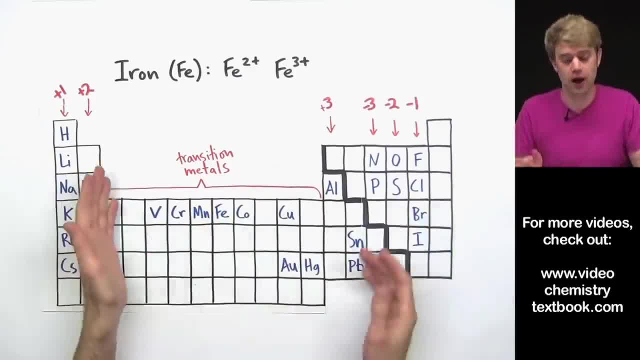 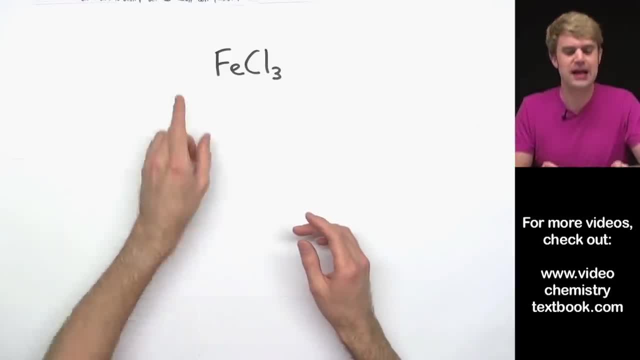 charges. some of them can even make four or five different ions, each with a different charge. so these different charges on transition metals really come into play when we want to name a compound that contains a transition. so here we have fecl3, and for the fe, the iron, we can't tell. 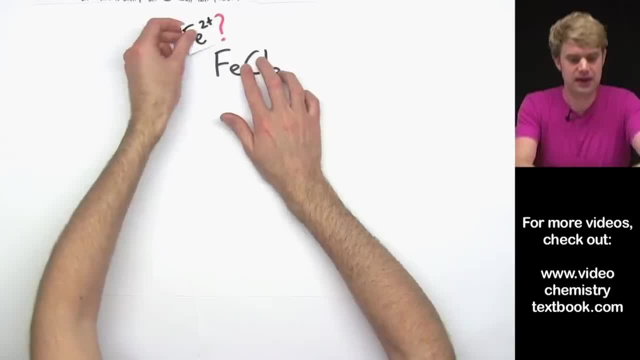 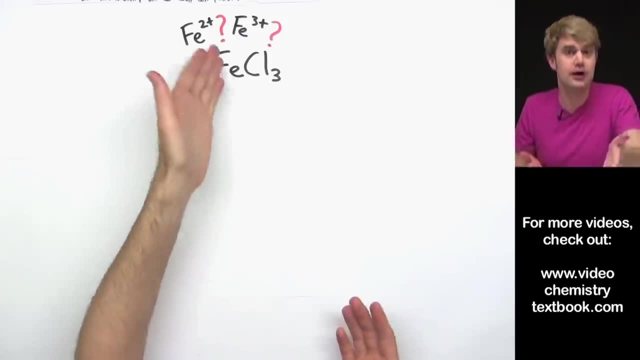 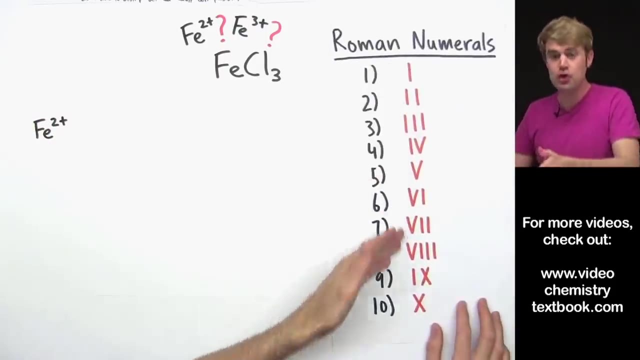 right away, just by looking at this, whether the fe is fe2 plus or whether it's fe3 plus. right, we have these two different types of ions that fe can make. now we can distinguish between these two ions by using roman numerals to give them different names. so the fe2 plus ion we call. 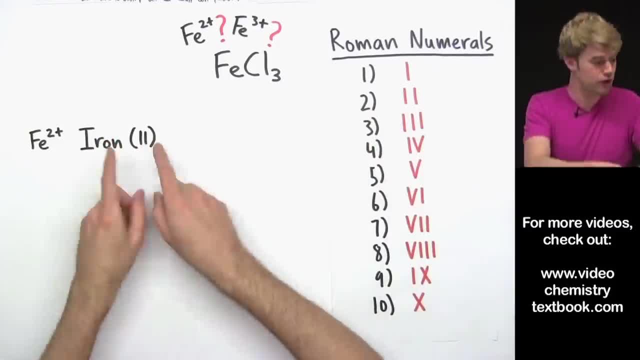 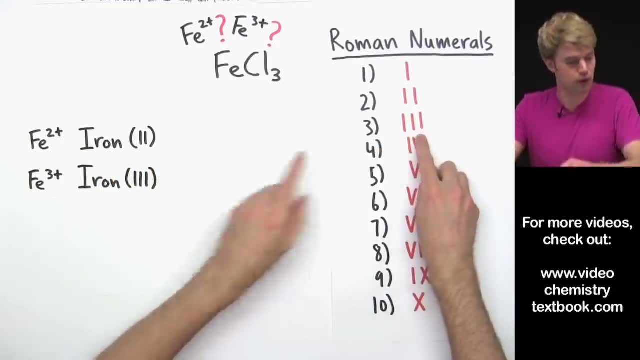 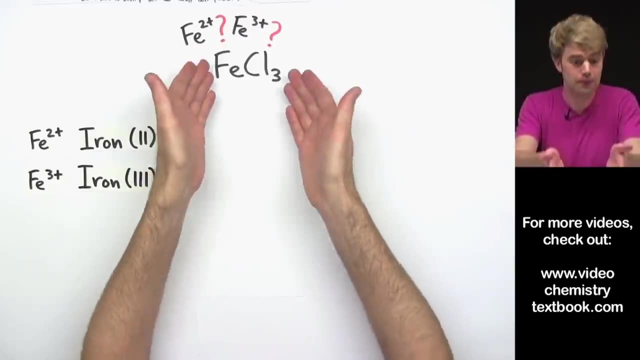 that iron two, with the roman numeral for two in parentheses the fe3 plus ion. we call that iron three, with the roman numeral for three in parentheses, and we'll use these ion names when we want to name the whole compound. so if the fe here turns out to be fe2 plus, we'll call this: 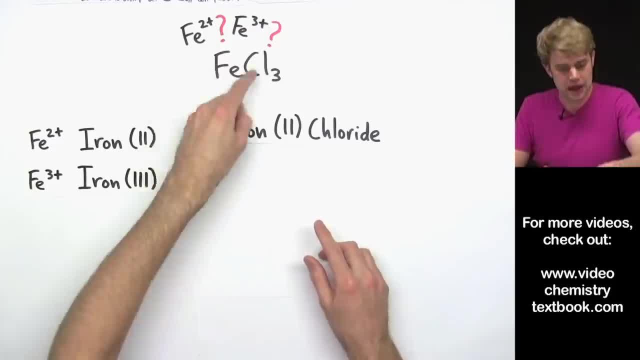 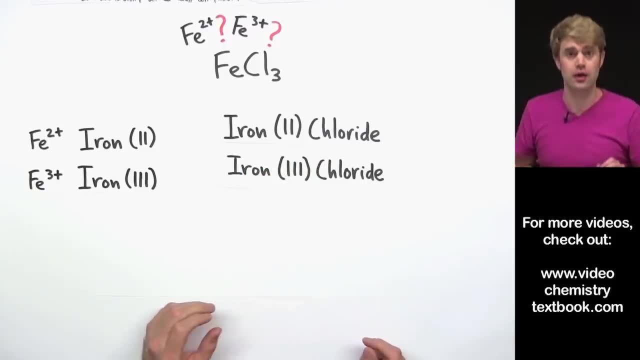 compound iron 2 chloride, and if this iron is iron 3 plus, we will call the compound iron 3 chloride. so in order to figure out whether we're talking about iron chloride or iron 3 chloride here, we got to do a little bit of math and work backwards to figure. 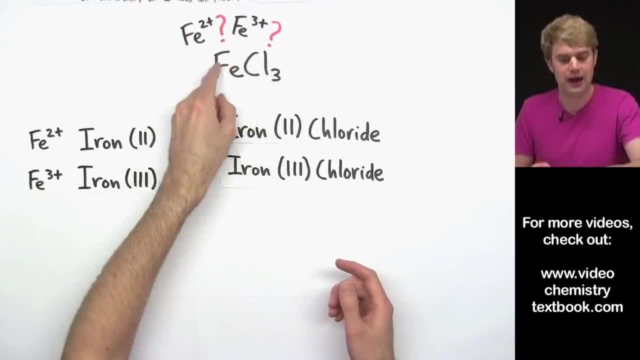 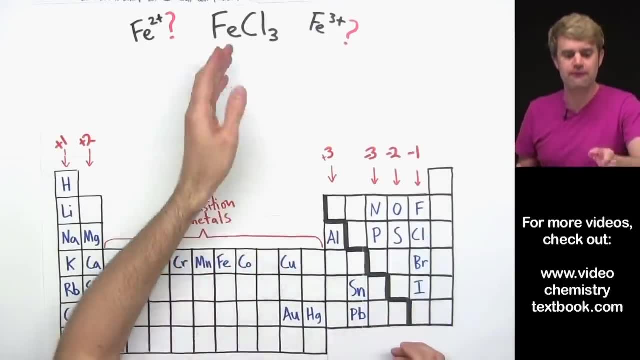 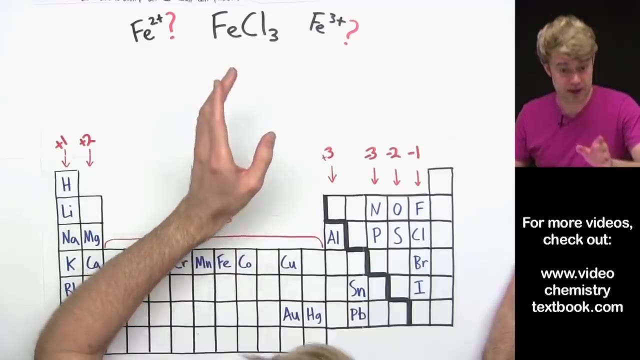 out which of these two charges iron has in this particular compound. let me show you how to do it. so, to find the charge of a transition metal, we start by focusing on the ion, with a charge that we do know, that's certain, that's not going to change, and for this that's going to be cl. 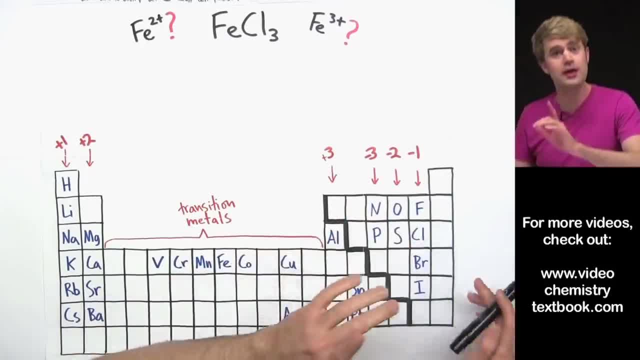 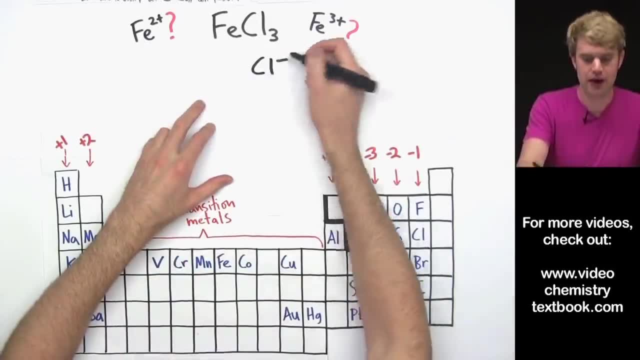 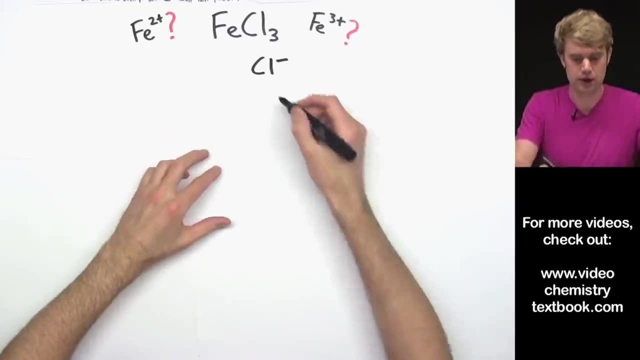 cl is in this column here on the periodic table, so that we know that in a ionic compound, cl always makes an ion with a 1 minus charge. okay, so we've got cl1 minus. now how much total negative charge do we have here? we have three cls, so that's going to be one. 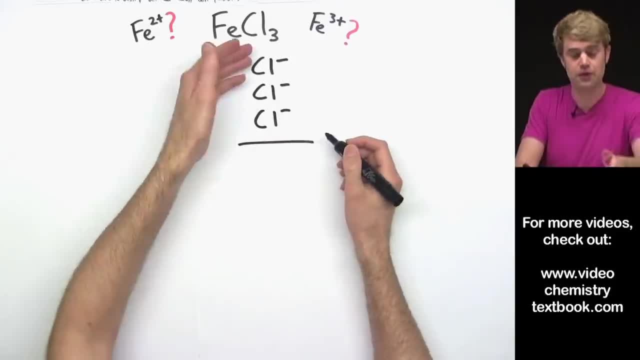 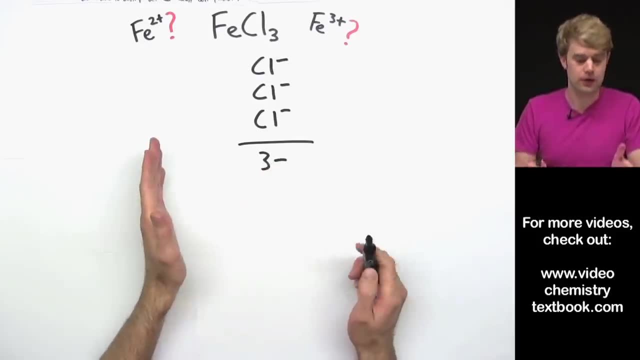 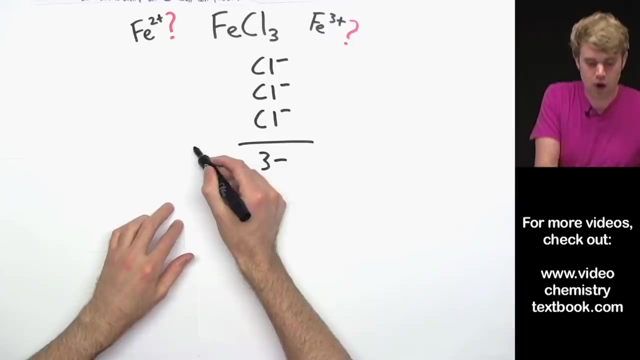 two, three, and since we have three of them, the total amount of negative charge is going to be three minus. now, in an ionic compound, the negative charge always has to balance out with a positive charge. so if we have three minus on this side, we've got to have three plus on this side. so 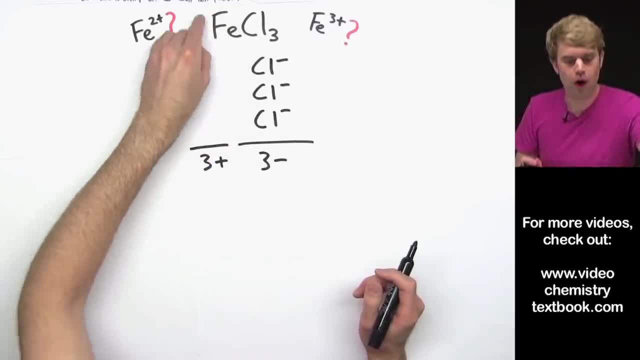 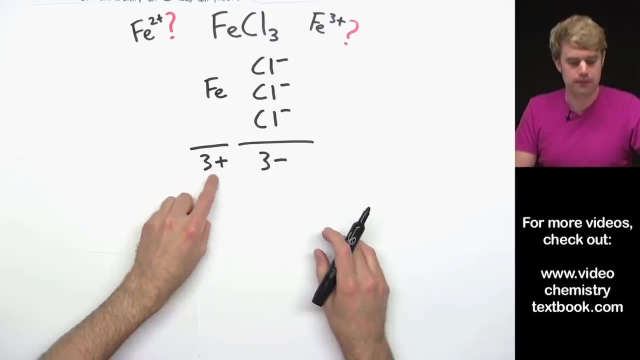 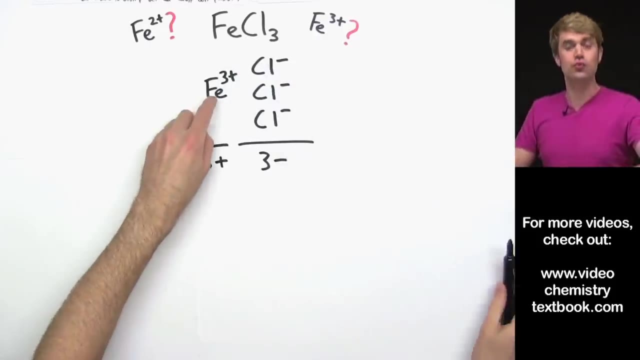 what's the charge on iron now? well, there is one iron ion in this compound, which means that all of the positive charge has to be on this one ion, which means that its charge is fe three plus. okay, three plus gives us three plus of charge, which has to be balanced out by the three minus over. 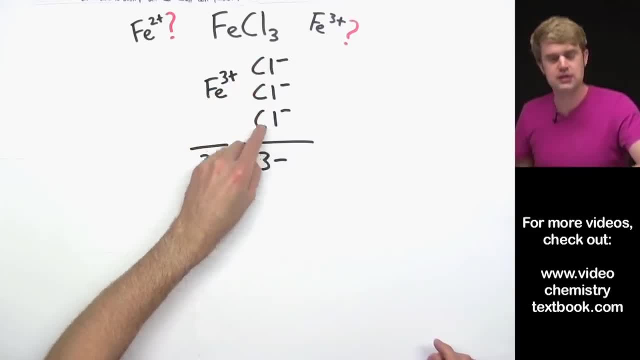 here, which is distributed over the three cl minuses. so that's how we figure out the charge on iron, and since this is iron three plus, the name for this compound is going to be iron three. and then for cl, when cl, when chlorine becomes a negative ion. 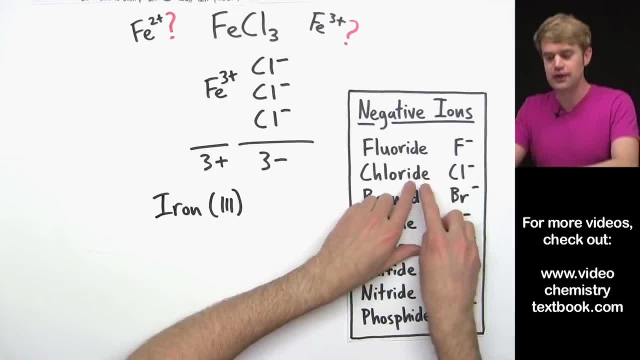 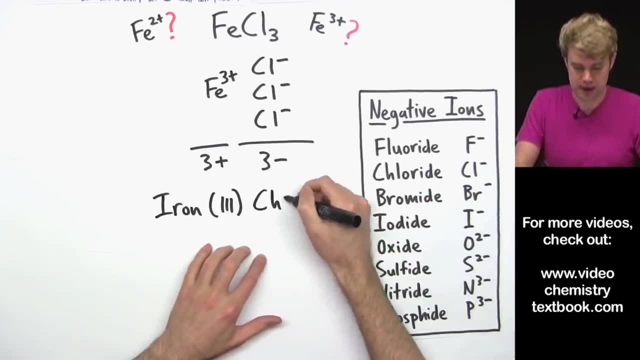 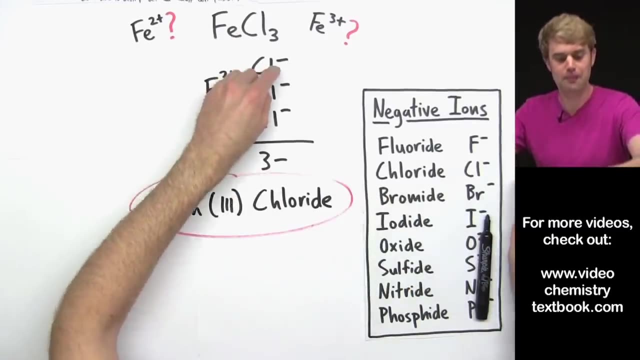 we call it chloride. the ide usually gets added to the name of an element when it becomes a negative ion, so chloride is what we call cl. one minus, so iron three, chloride is the name of this compound. we had to work backwards and figure out the charge of iron and then we can call it iron three. so if 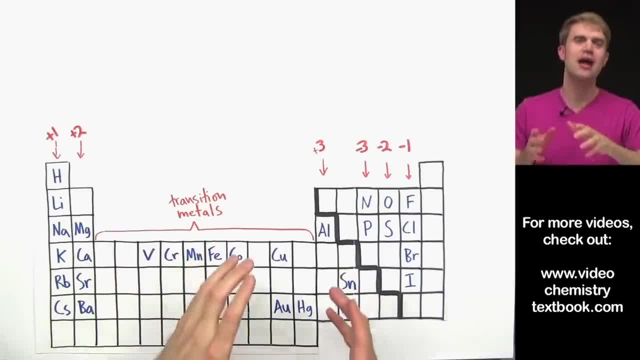 you want to get really good at naming compounds with transition metals and using the roman numerals and all that. you've just got to get a lot of practice. so i've made another video. that's just a whole bunch of practice problems on naming ionic compounds with transition metals. but before you check that out, i want to talk about a couple of 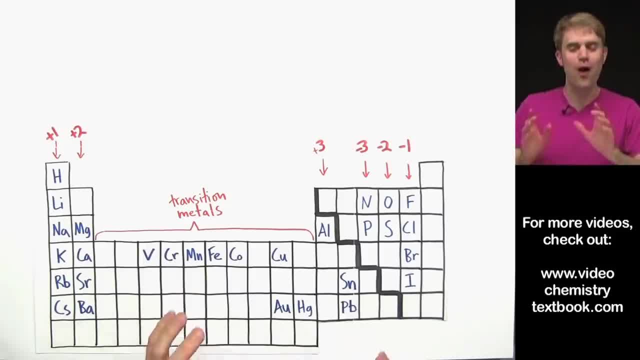 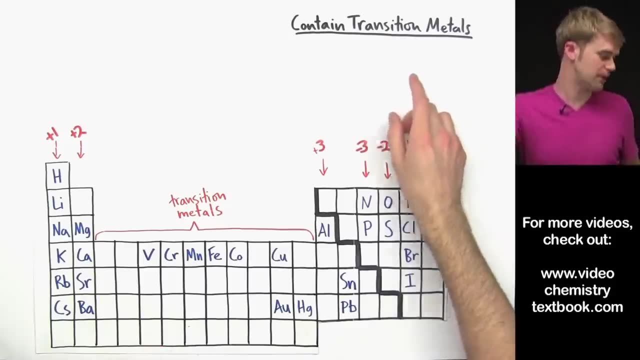 important things. the first thing i want to talk about is when we use roman numerals for naming and when we don't. this confuses a lot of students, okay, so when do we use roman numerals? well, we use roman numerals when we're naming compounds that contain transition metals. so 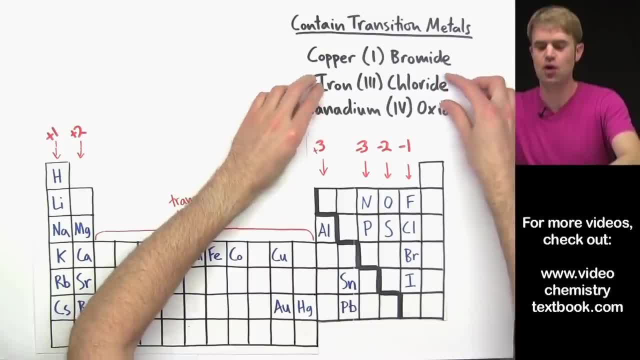 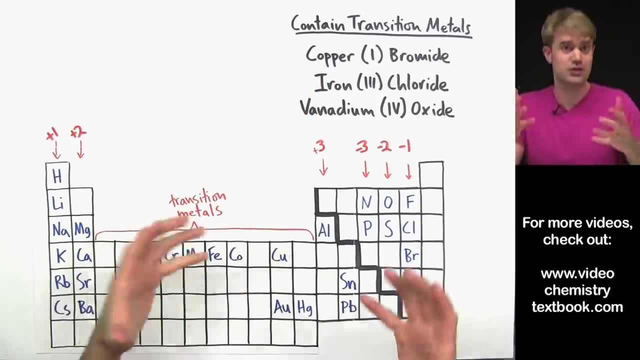 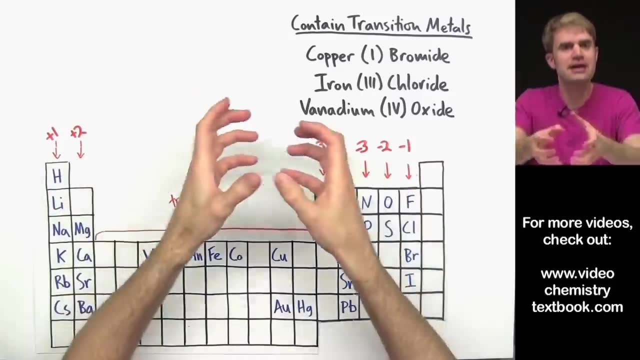 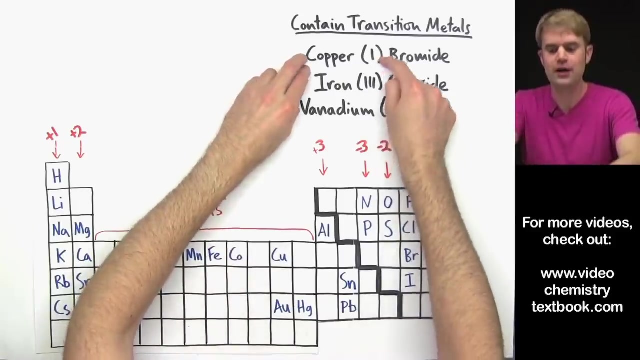 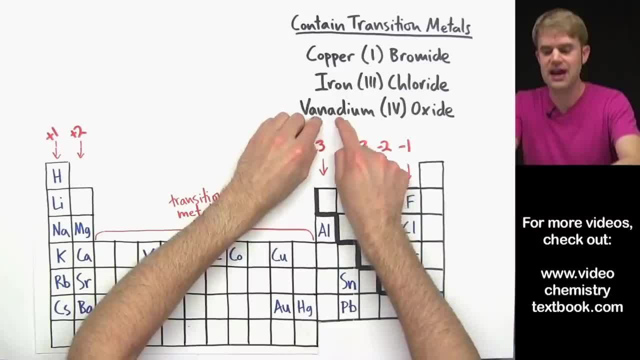 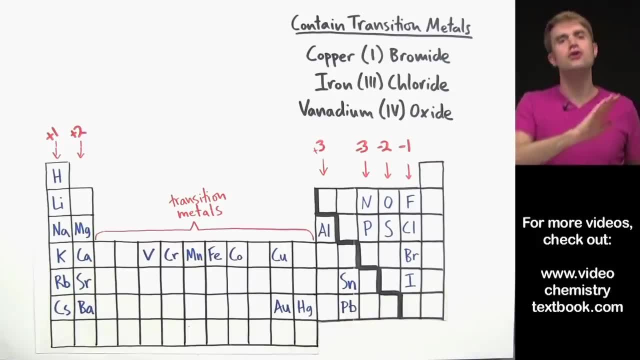 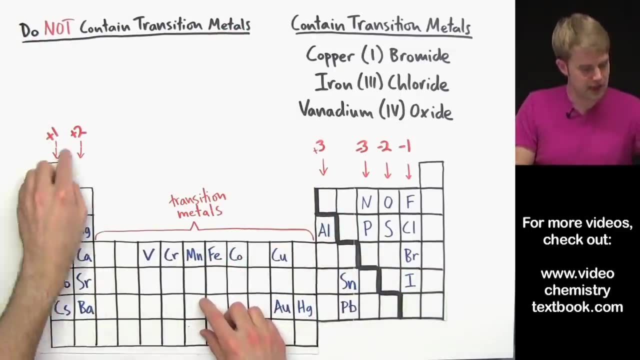 cl2, iron 3 plus. here we're talking about vanadium 4 plus, because they could be a variety of different ions. now, on the other hand, we don't use Roman numerals when we're naming compounds that don't contain transition metals, that contain, for example, the metals over here. take potassium iodide, for example. potassium. 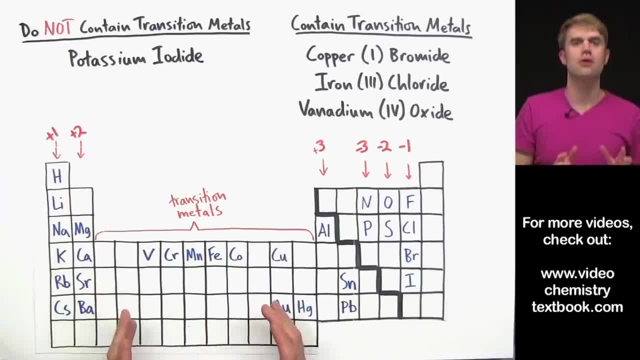 K is in this column. it's in the 1 plus column, which means that in an ionic compound, potassium always makes an ion with a 1 plus charge. that's the only choice. it can only be 1 plus, so we don't need to put a Roman numeral in there to. 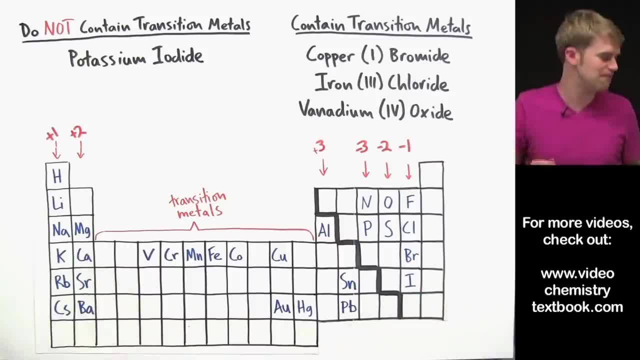 specify that it's 1 plus, because that's the only choice that it could be calcium nitride over here. calcium is in this 2 plus column and it can only make an ion with a 2 plus charge in an ionic compound. so again, we don't need a Roman. 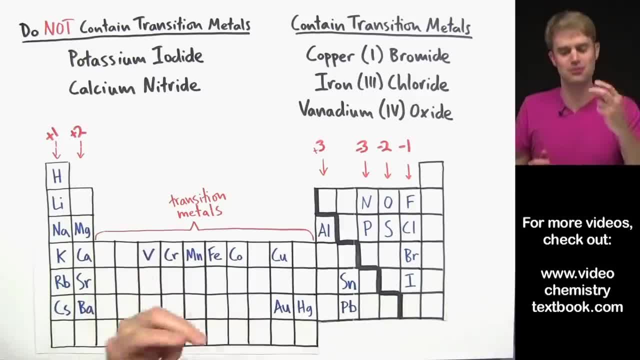 numeral to say that, because there's only one choice, and that's 2 plus. now aluminum over here can only make a 3 plus ion, so you don't need to use Roman numerals with aluminum either, and I should point out that some of these metals here that are not technically transition metals still can make ions. 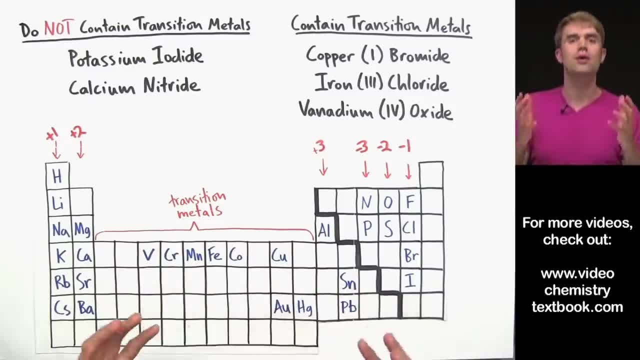 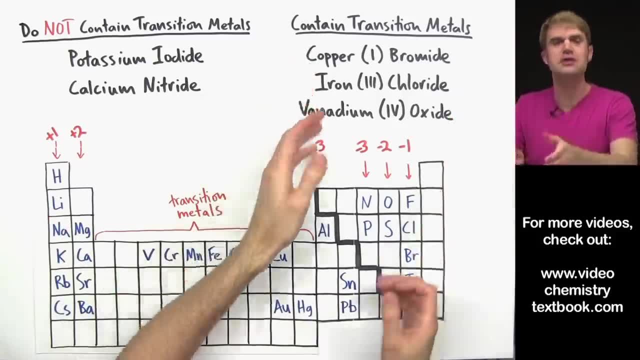 with different charges. so we have to use Roman numerals when we name compounds with tin and lead in them as well. but here's the big point: if you're naming compounds with ions that can make different charges, you always need the Roman numerals. but don't put those Roman numeral in the column. you're simply going to be using 2 plus ions. 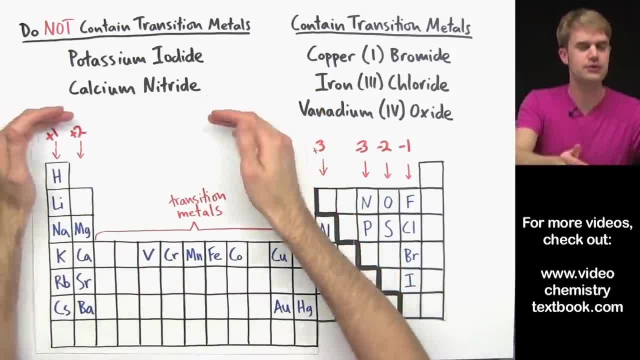 you're going to be using two plus ions now. aluminum over here can only make a 3 plus ion. numerals in if you're naming compounds with metals that can only make one charge. Not only is it a waste of time to put those Roman numerals in, but it's wrong. 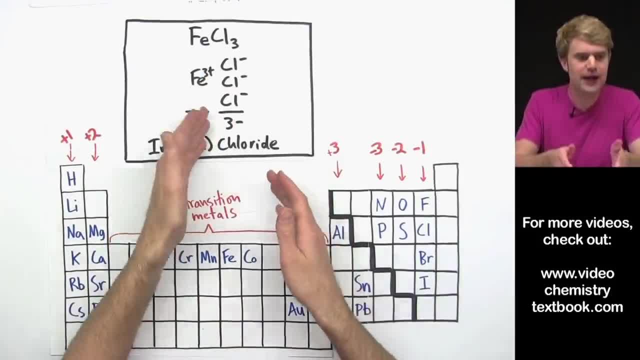 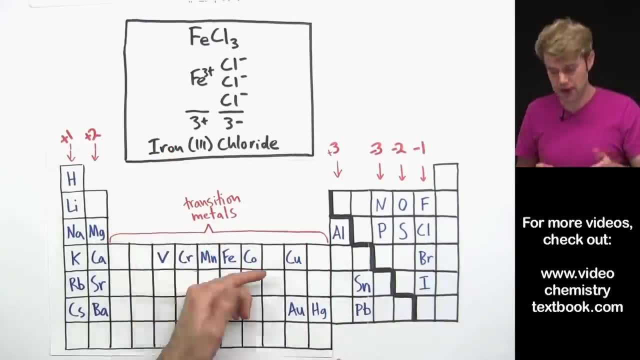 You just shouldn't put them in there Now. we have to use this method of working backwards in order to name compounds that contain most transition metals, and we also have to use this method to name compounds that contain metals like tin or lead that are able to make more than one type of ion. 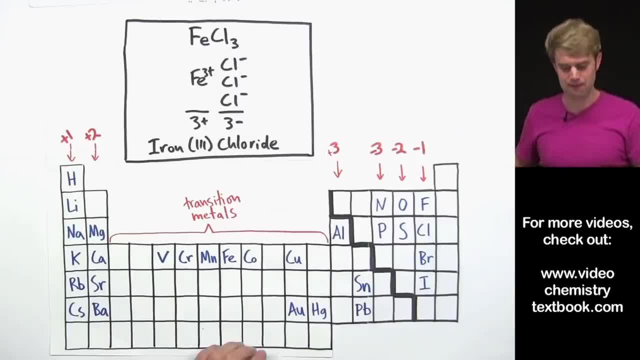 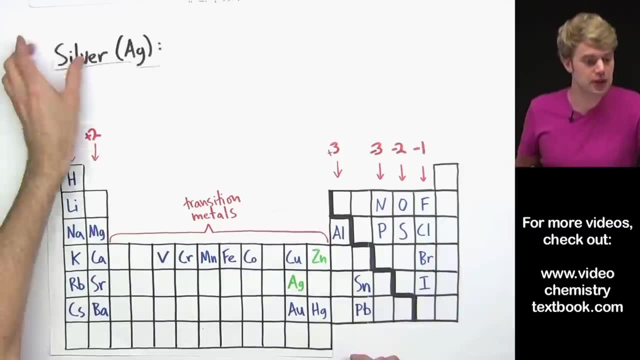 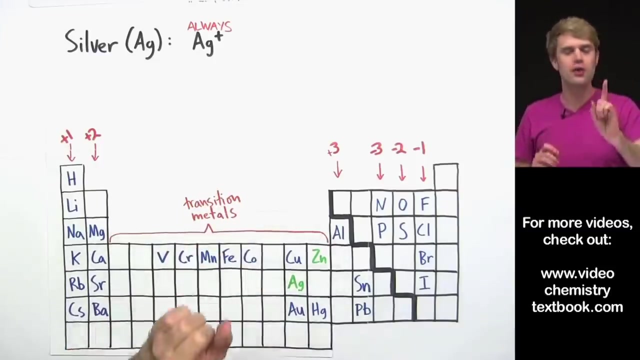 But there are two important exceptions that I need to tell you about, and these are silver and zinc. Even though these two elements are transition metals, they're only able to make one type of ion, So silver always makes Ag. It's always one plus and only one plus. 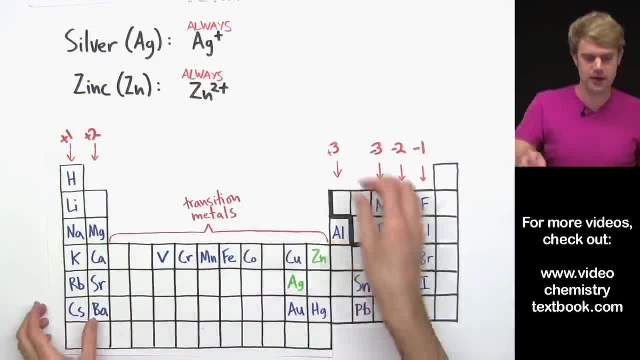 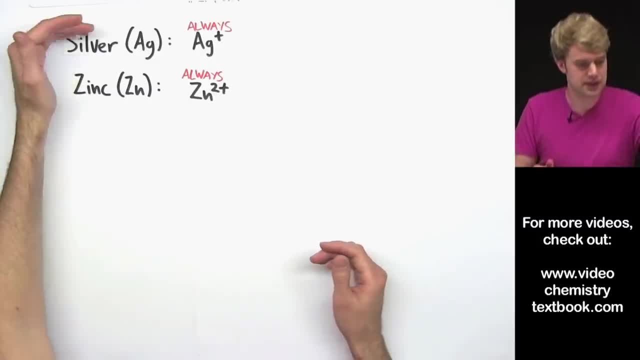 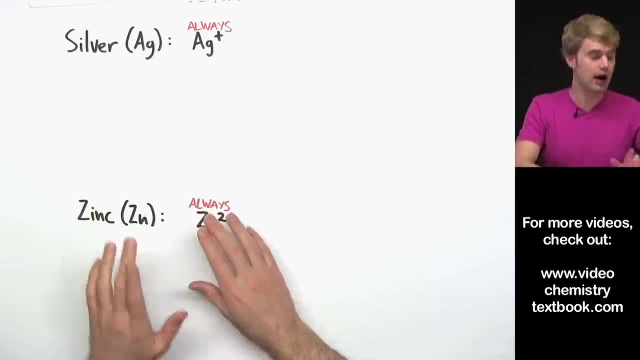 Zinc always makes Zn. Silver always makes an ion that is Zn. Now that means that when we name compounds that contain silver or zinc, we don't have to use Roman numerals, because we're only talking about one type of ion, So a compound like this, AgCl. you don't have to do any math at all. 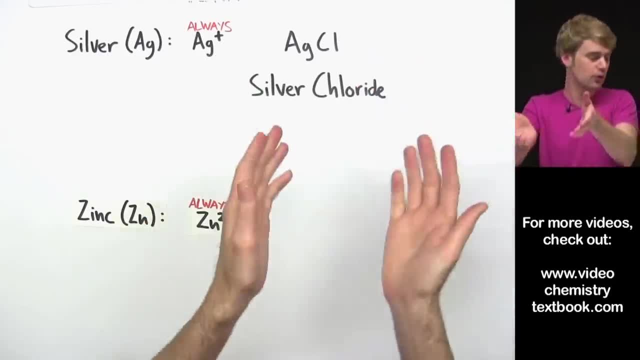 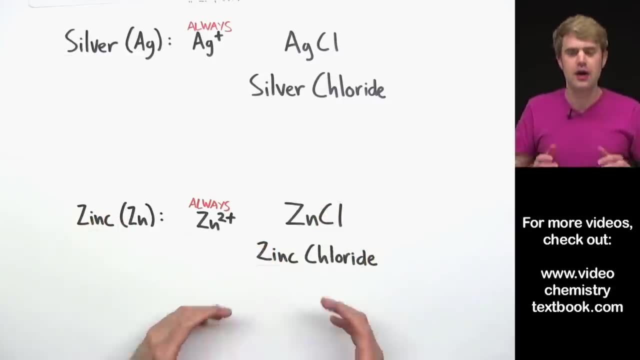 You don't have to use a working backwards approach. You just call it silver chloride ZnCl here. super easy. We just call that AgCl ZnCl, And since these elements always make ions with just one charge, we don't have to use 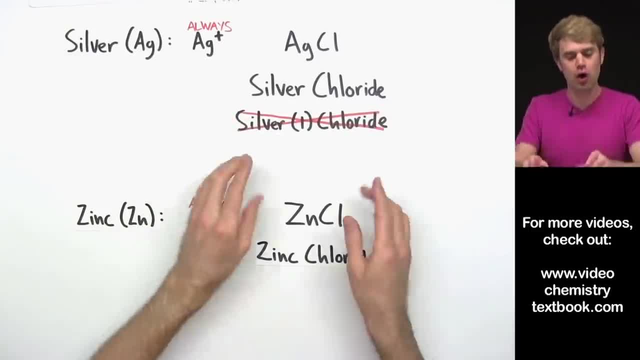 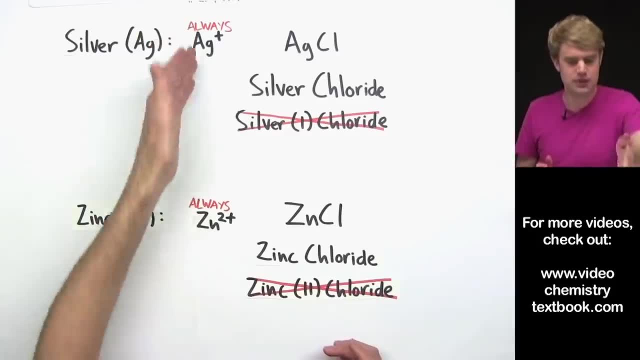 the Roman numerals when we're naming them. So it would be wrong to call this silver chloride or ZnCl. here There's only one possible ion, so we don't use the Roman numerals. We only use the Roman numerals if we're trying to distinguish between multiple types of ions. 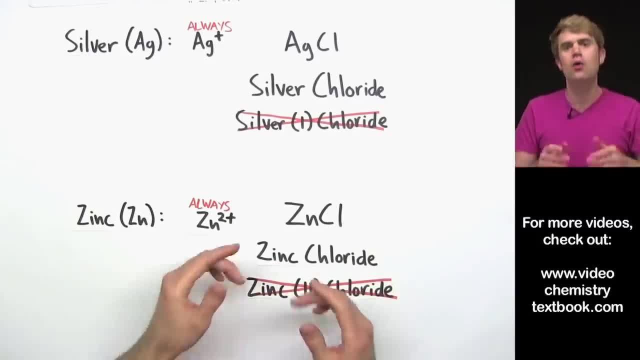 with different charges. So that's the introduction to how we name compounds that have transition metals in them. In the next video we'll do a whole bunch of practice problems so you can really get the hang of it. This is one of the things that you just get better and better at with more practice. So check out that video. You'll get super good at it really fast.